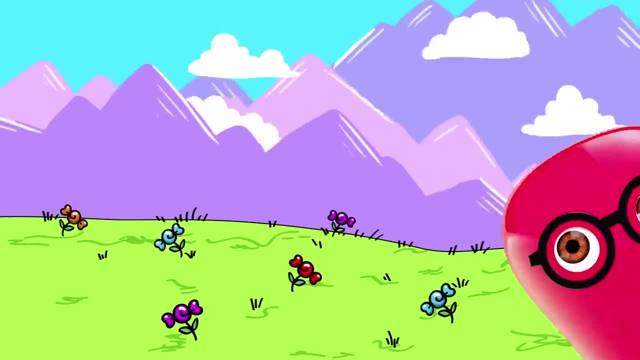 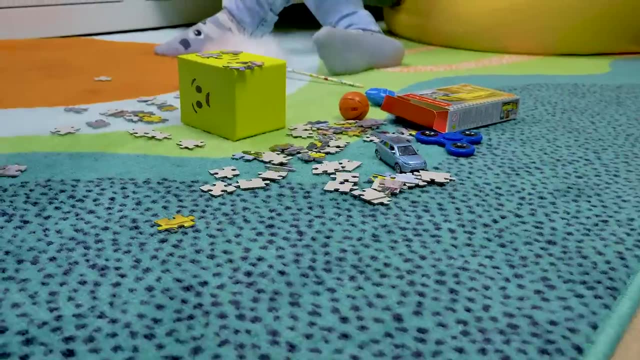 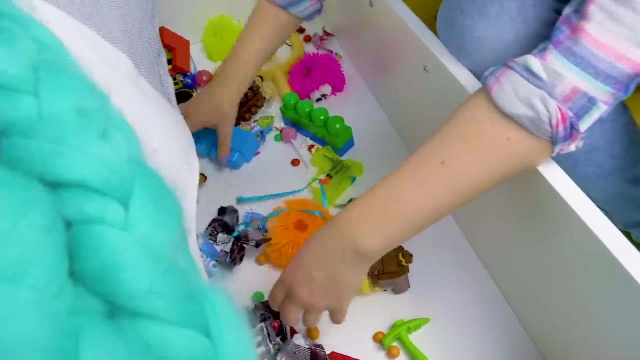 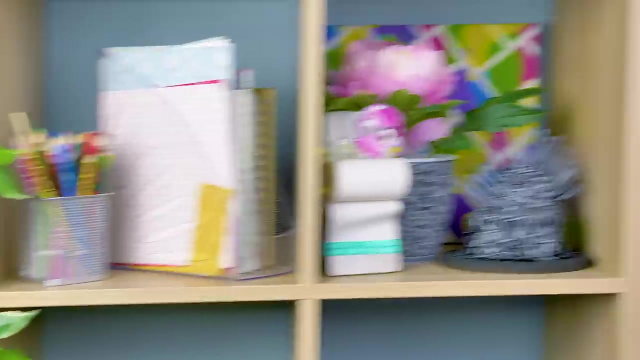 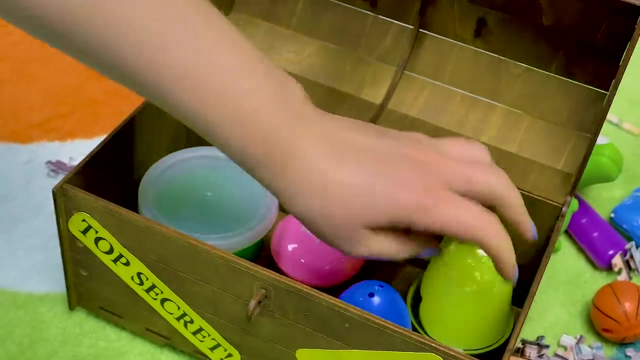 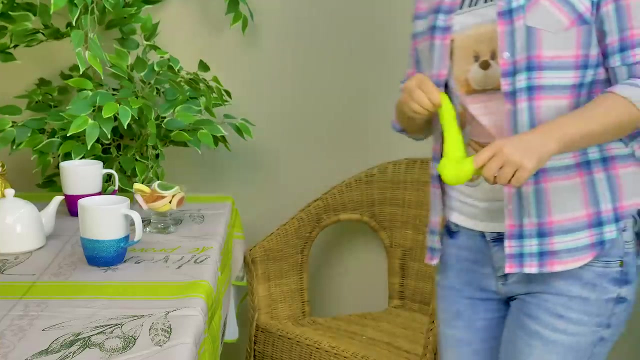 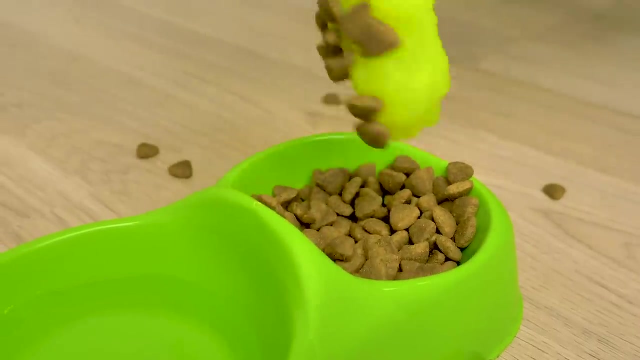 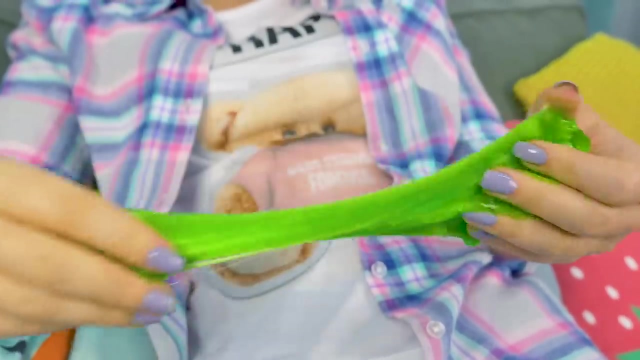 Nope, Okay, Where is it? I know that clever slime keeps his slime collection somewhere in here. Hmm, let's see. Aha, Now I'm gonna have a real blast. Woo, Oh, oops, Oh, ew, Ah, okay, Mm-hmm. Ah, this is so relaxing. Oh, yeah, Oh, what is this? 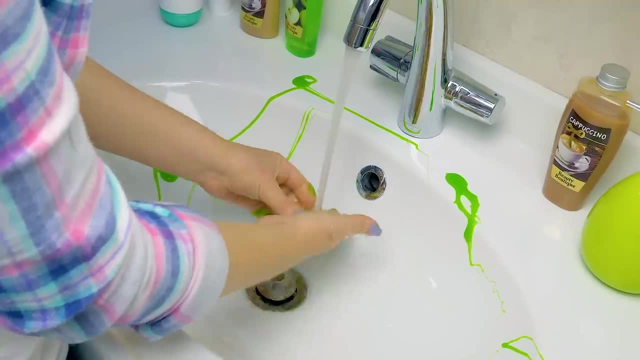 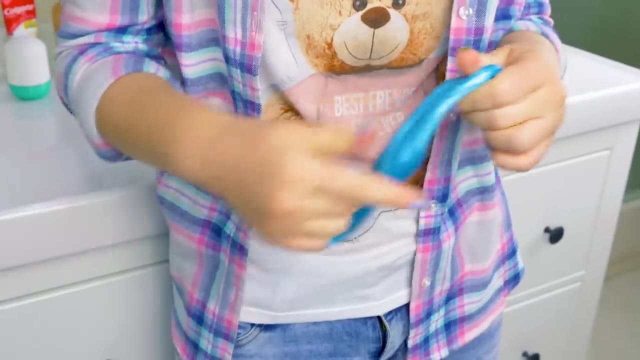 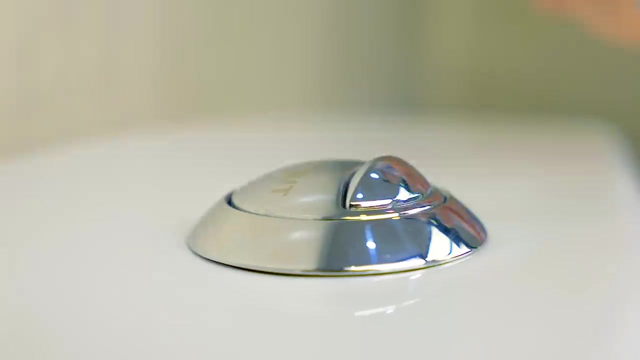 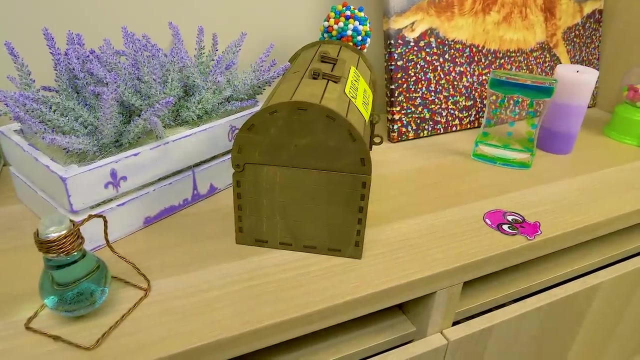 Ew, Ah Okay, let's try this one. Hmm, What, Oh no, Ah well, I've got more slimes in stock. What No more left? Fine, he'll do without them. Right Today I need. 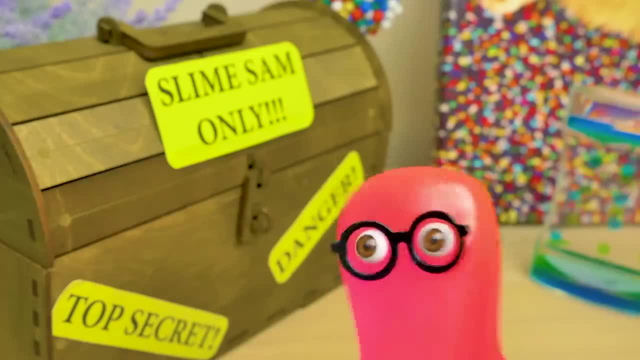 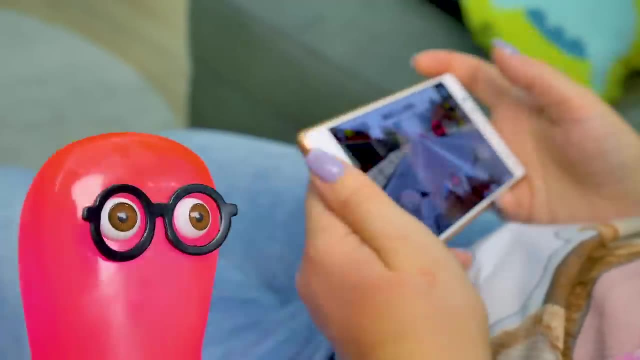 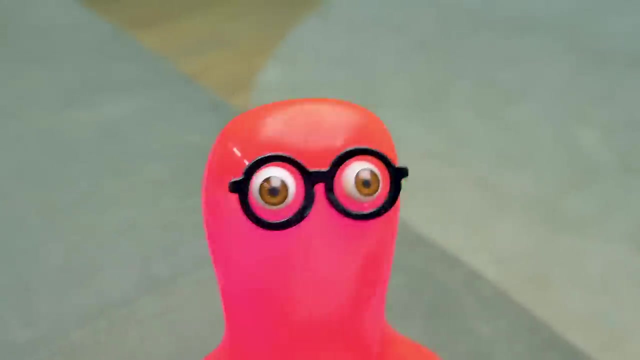 What, What, What's this? What, Uh, where, Oh, oh, oh, no, Samantha, Hey, I'm talking to you. Why all the yelling? Why is it empty? Who knows? I know it's you. Give me my slimes back. 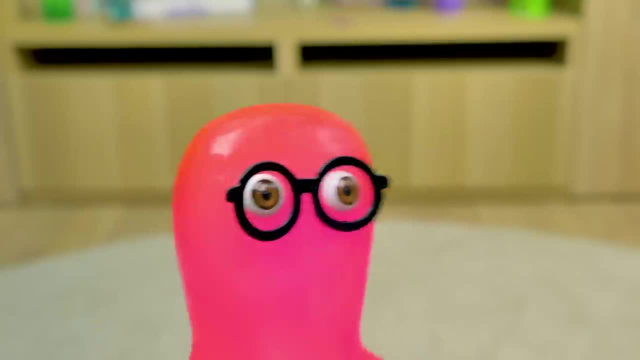 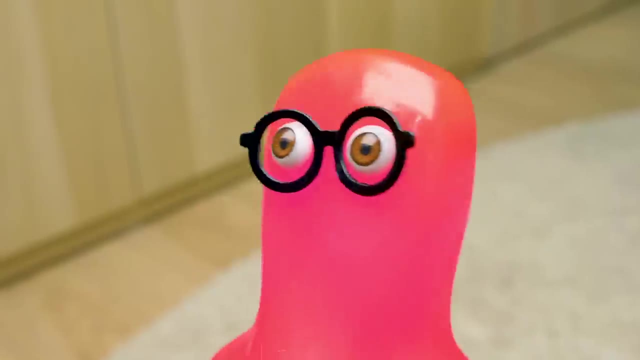 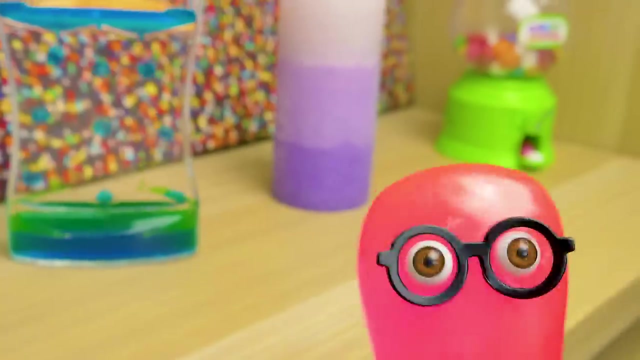 Get lost, Sam. Your slimes are all gone. What Ow Simple, I demand compensation. Ugh, why are you so annoying? Because slimes are my. Slimes are my everything. They are more precious than candies. Chill out, Sam, I'll make you a hundred slimes. 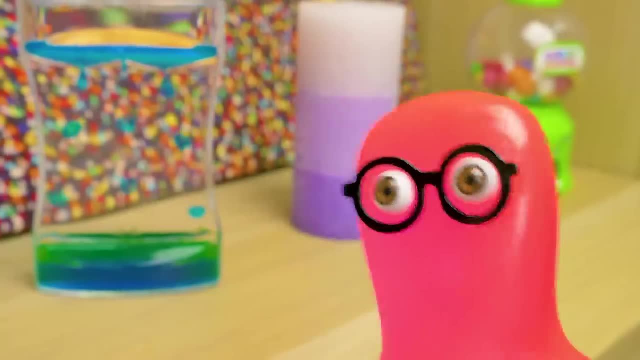 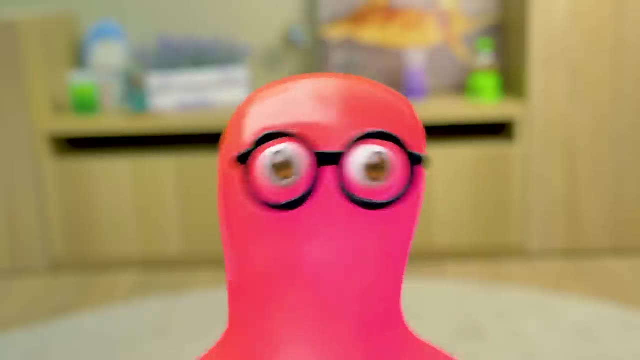 A hundred slimes. But no way, Sue spends lots of time eating with one slime and you say a hundred. Yeah well, she doesn't know my secret. Oh well, I'm waiting. You wait when pigs fly, Hey. 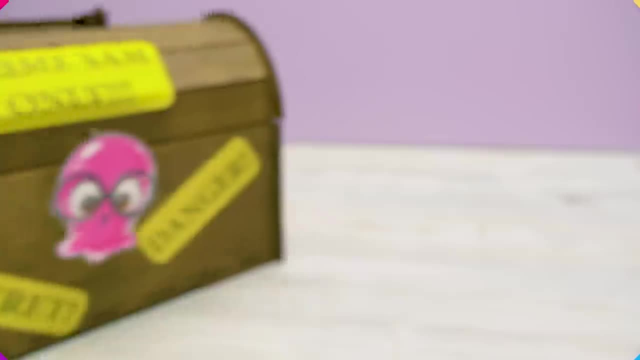 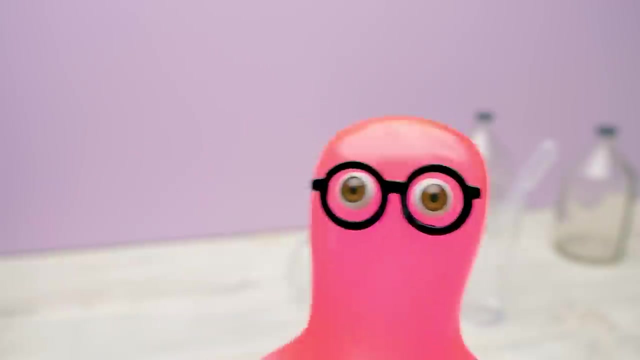 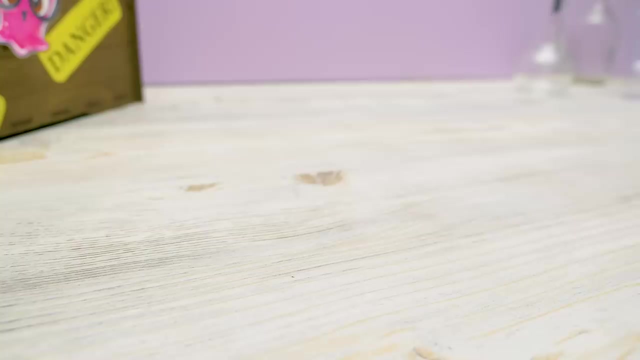 Fine, fine, I'm going. Hey guys, Today, Samantha will show us how to make a slime in 30 seconds. I find it hard to believe, but we'll see. How long does it usually take you to make a slime? Pause the video and write in the comments. 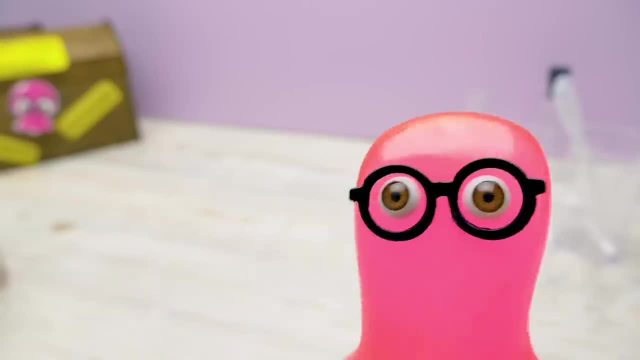 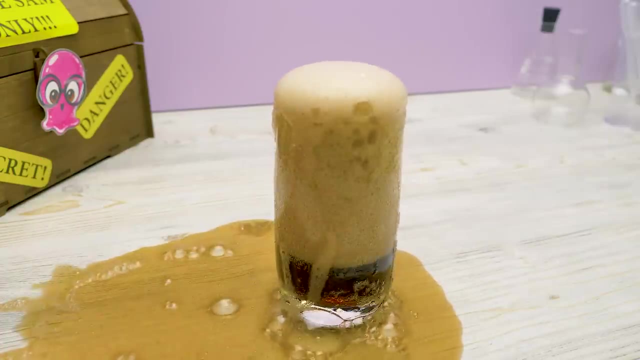 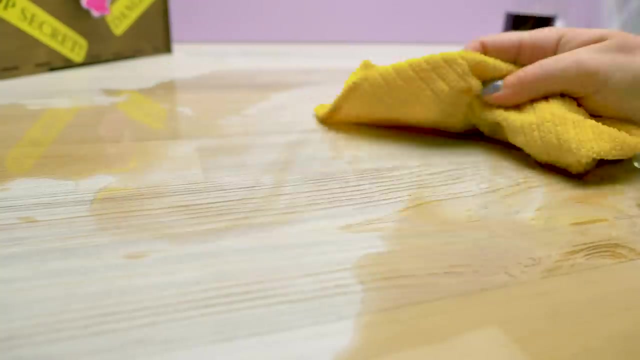 Ah, where is she? Do I always have to wait? Samantha? Never fear, Samantha is here. Oh careful much. Oh sorry, your slime mess. We are going to make slime and everything will be a mess. Nope, this recipe is famous for no mess. 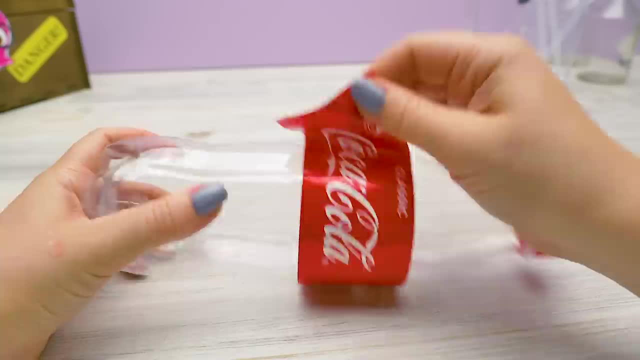 Hmm, this recipe seems cute. Hmm, this recipe seems cute. I'm more curious and curious. Listen, why is nothing ready yet? What do you mean? It's your recipe, As if you didn't know what slime is made of. 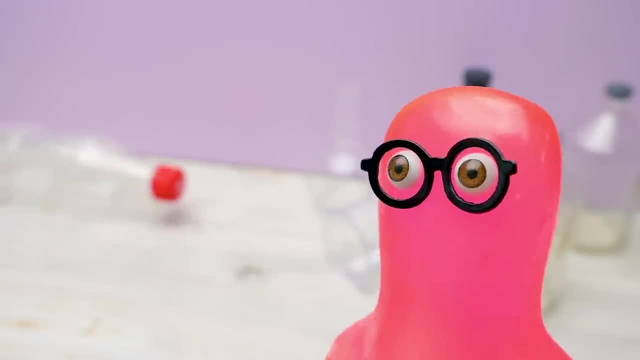 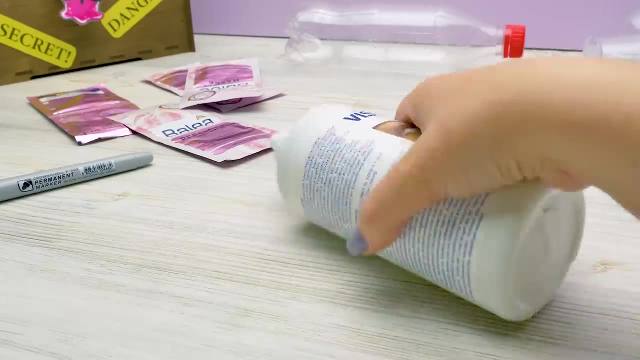 Right, I'm off. Hey, hey, hey, hey, Scared, eh Gotcha. We'll also need a marker, some face masks- by the way, these were mine- a bottle of contact lens solution and some baking soda. 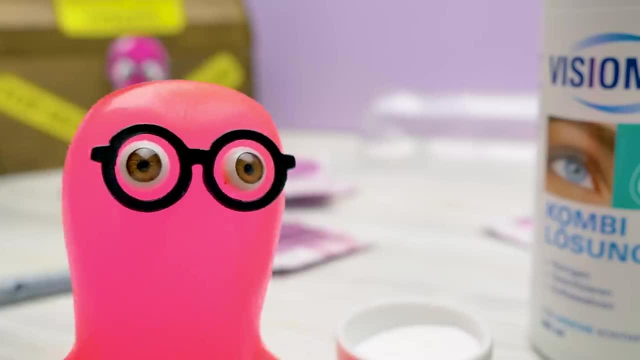 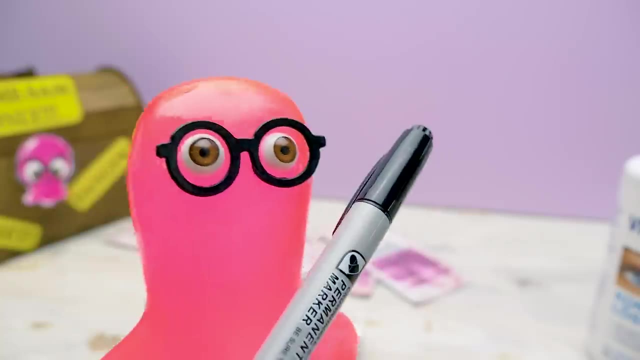 These items are quite suspicious. Are you sure it'll work? I've tried it before. stop panicking. First of all, let's make a measuring cup out of a bottle Slime marker. Here's your marker. oh, slime maker Samantha. 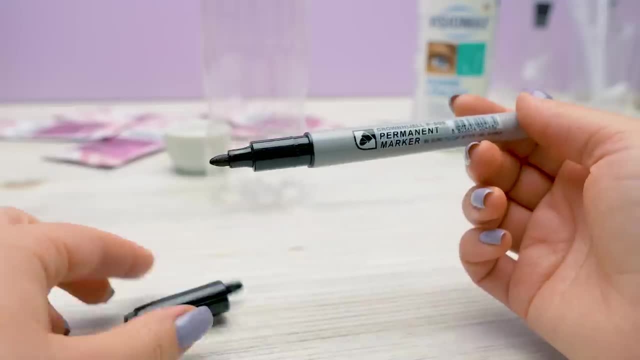 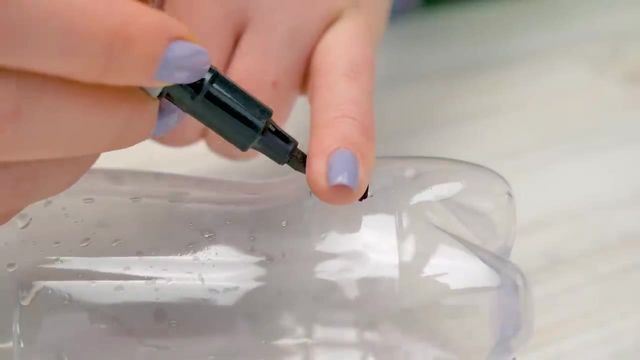 If you keep teasing me, I'm not making it Zipper on my lip. That's better. Let's make two markings on the bottle: Two fingers high and one finger high. This will be a guideline. The first ingredient is the face mask. 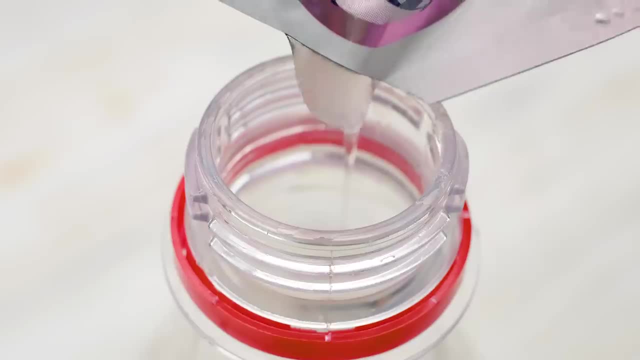 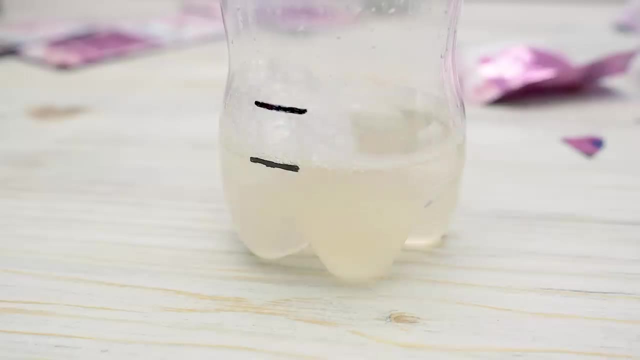 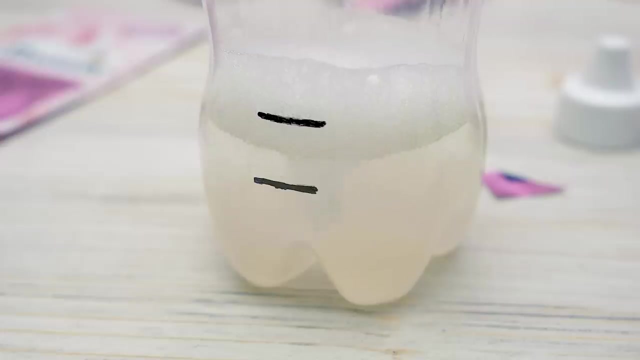 It's almost as relaxing as playing with slime. Now let's add some water. The first mark is the guide here. Aha, good, Now let's add contact lens solution. up to the second mark There. What do you think? Which sister wears contact lenses? Write in the comments. 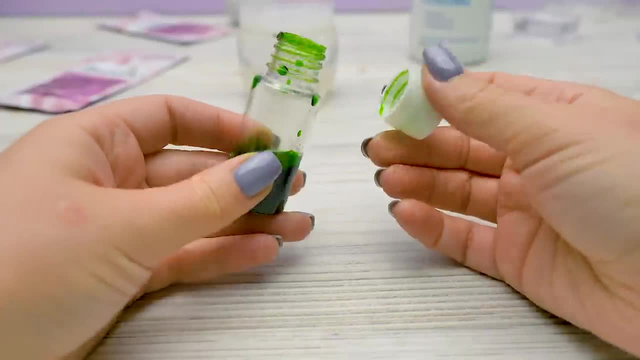 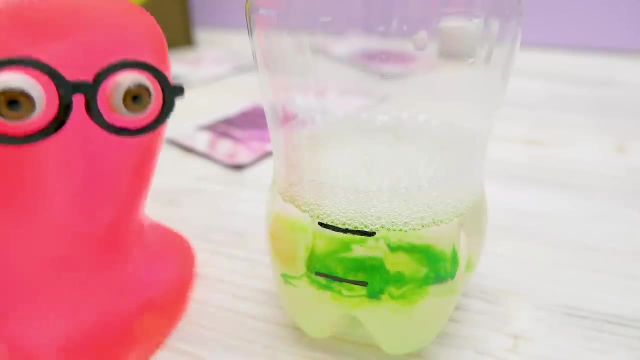 Boom, boom, boom, boom. I've almost forgotten about one of the fun ingredients: coloring. Let's add a few drops. Phew, I thought it would be a pale slime. Nope, it won't be now. And the last ingredient: baking soda. 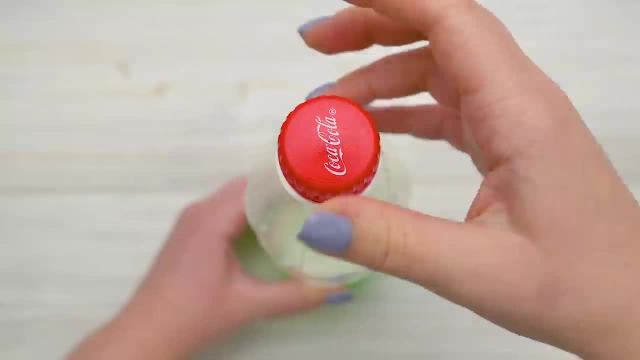 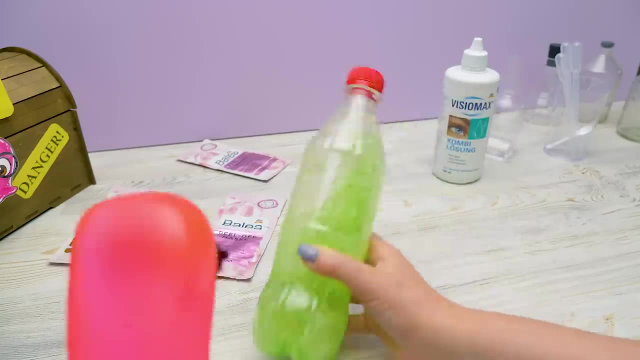 Hey, you said no mess, Just a few specks of soda. But now bottle shaking time. We need to shake the contents really well until we get the slime consistency Very fast. Your bottle shaking makes me dizzy. Well, sit down.